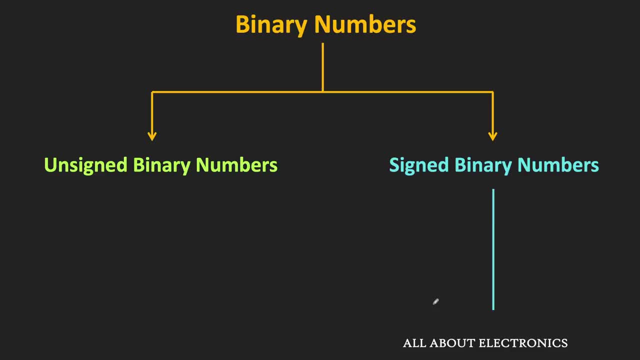 So there are 3 different ways to represent this signed binary number, That is, signed magnitude form 1's complement and the 2's complement. So, one by one, we will see all 3 different types of representations And to understand them more clearly, let's briefly talk about the unsigned binary numbers. 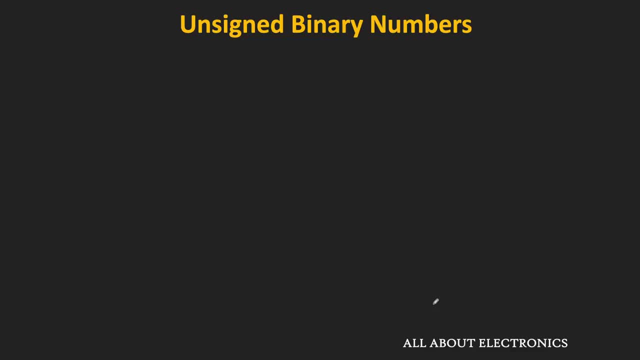 So, as I said earlier, Using this unsigned binary number representation we can represent only positive numbers. So if we have a n bit of unsigned binary number, then all n bits are used for representing the magnitude or the value of that binary number. For example, if we represent 16 in the unsigned binary number, then all 5 bits are used for. 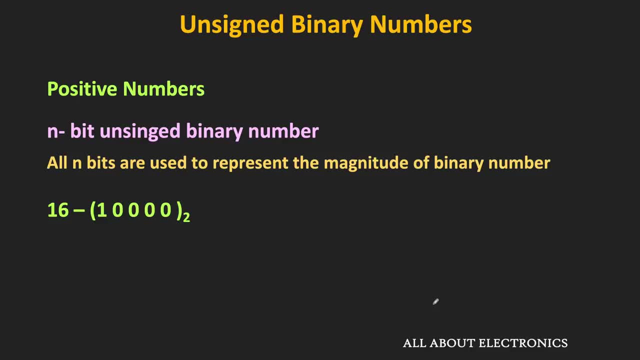 representing the magnitude of that number. So in this unsigned binary number representation, the n bits, the range of numbers which we can represent are from 0 to 2 to the power n minus 1.. For example, using 4 bits we can represent the numbers starting from 0 to 15.. 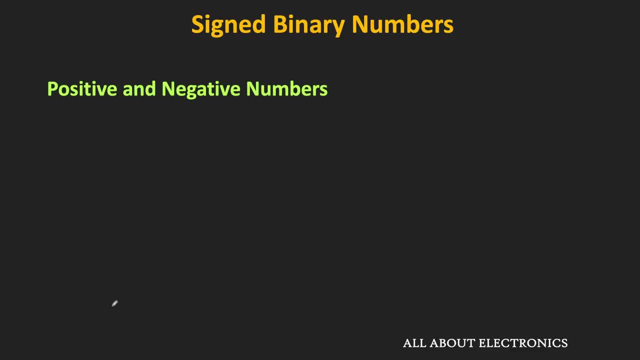 On the other hand, with the signed binary numbers we can represent both positive as well as the negative numbers. So in this signed binary numbers the most significant bit, or the MSB, is the signed bit. So if we have a n bit, then all n bits are used for representing. the magnitude or the value of that binary number. So in this unsigned binary number the most significant bit, or the MSB, is the signed bit. So if we have a n bit, then all the Brown の 7 is used for representing the magnitude or the value of that binary. 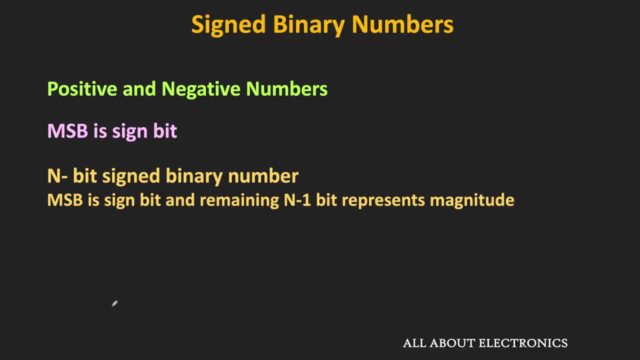 number For masternashray. we need to substitute n And we also need the 1.. So we need to substitute n And if the N is not inside this unsigned binary number, then the MSB is the signed bit R can be. 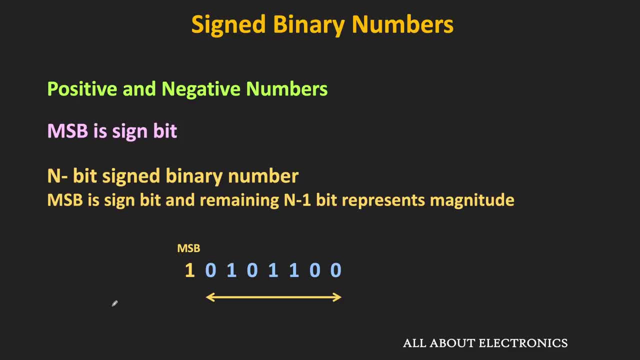 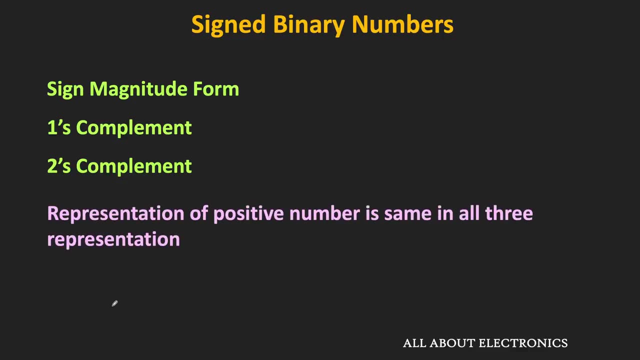 used to represent this magnitude or the value of that number. So depending on the value of the signed bit, we can decide whether the number is ground, binary number ie sine magnitude, form 1's complement and 2's complement. So in all three forms the representation of the positive number is same. 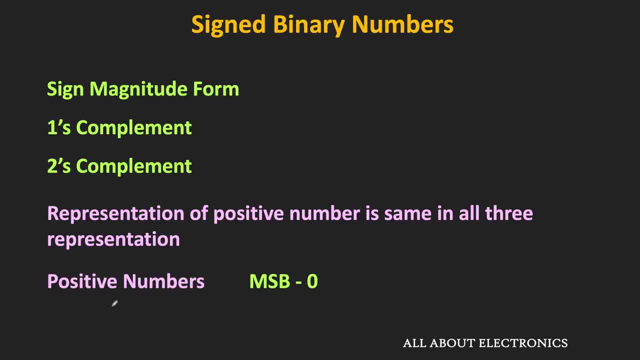 So for the positive number, the sine bit or the MSB is equal to 0,, while for the negative number, this sine bit is equal to 1.. Now, although for the negative numbers, this MSB or the sine bit is 1 in all these 3 forms. 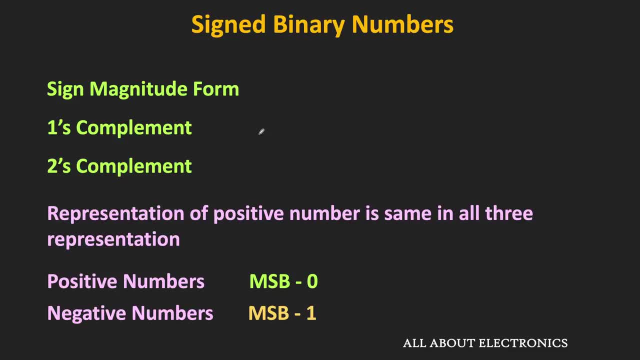 but if we see the actual number representation, then it is different in all these 3 forms. That means, suppose, if we represent the same negative number in the sine magnitude form or in 1's complement and 2's complement form, then their actual representation is. 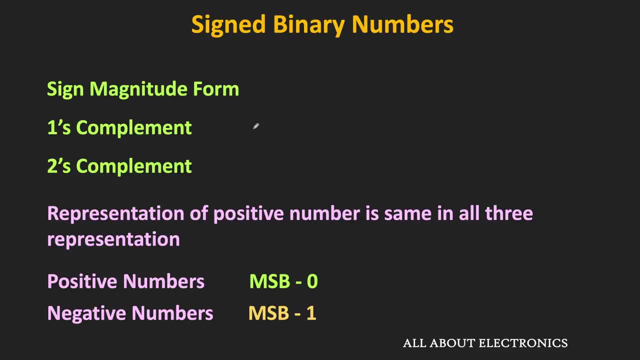 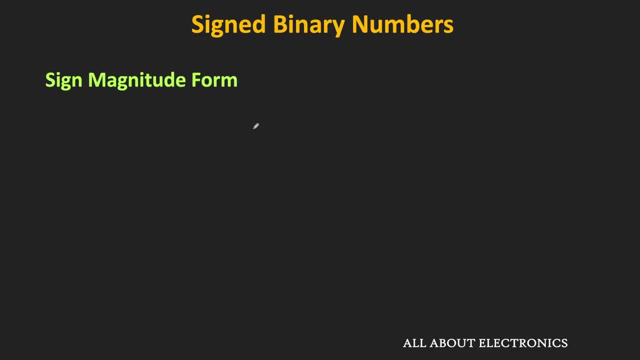 different in all 3 forms. So one by one we will see that how to represent the negative number in all these 3 forms. And first let's start with the sine magnitude form. So this sine magnitude form representation is pretty straightforward. 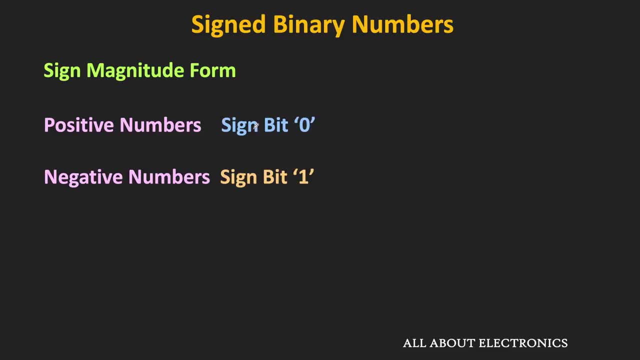 So for the positive numbers the MSB or the sine bit is 0,, while for the negative number this MSB or the sine bit is 1.. And the magnitude of the number is represented in the true binary form. For example, if we represent this plus 34 in a 8-bit sine magnitude form, then its magnitude 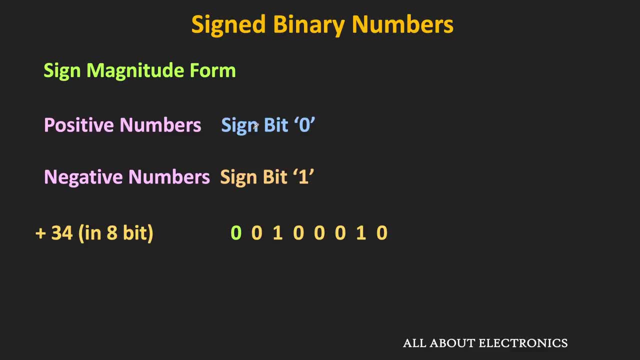 is represented in a true binary form, while a 0 is put at the MSB, On the other hand, for the minus 34.. Instead of 0. There is a 1 in the sine bit, But if we see the magnitude representation then it remains the same. 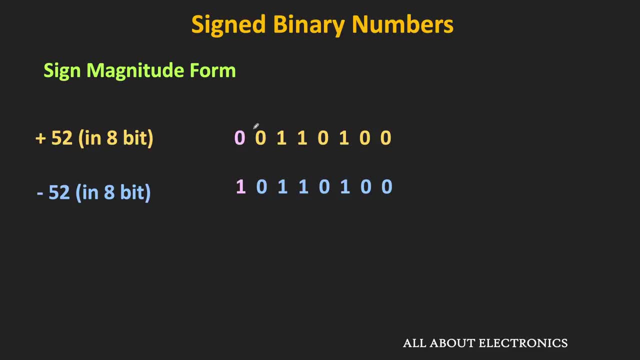 So let's take one more example. So if we represent the plus 52 in a 8-bit sine magnitude form, then the MSB is equal to 0 and in the remaining 7 bits the magnitude of the number is represented in the true binary. 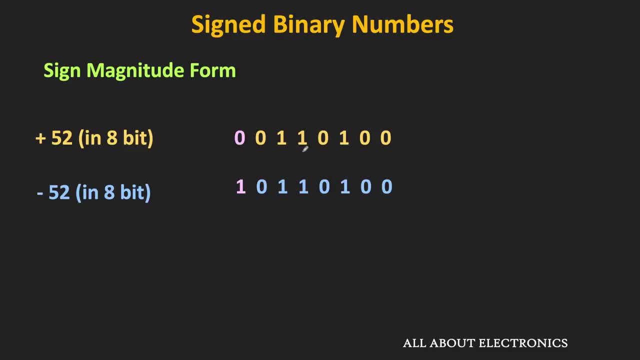 form That is equal to 0, 1, 1, 0, 1, 0, 0.. On the other hand, if we represent the minus 52 in this sine magnitude form, Then this MSB, or the sine bit, is equal to 1.. 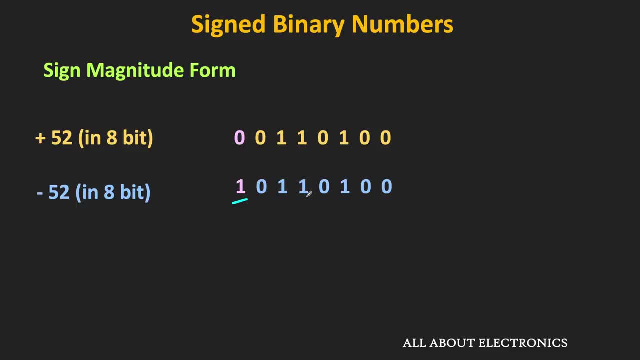 And if we see the magnitude bits then it remains the same. So that is how we can represent any sign binary number in this sign magnitude form. But there is a special case of representing the zero in the sign magnitude form. So in a sign magnitude form there are two different representations of the zero. 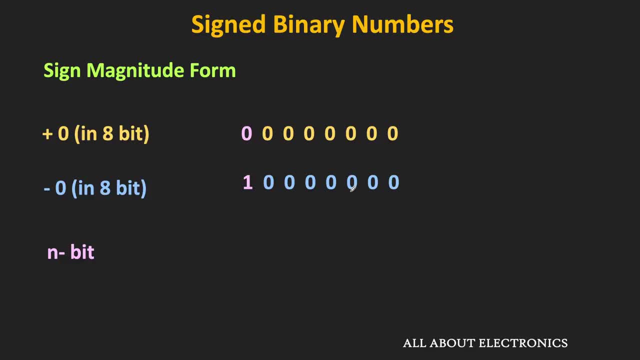 So in this sign magnitude form, using the n bits, The range of numbers which can be represented in the sign magnitude form And the magnitude of the numbers which can be represented in the sign magnitude form. numbers which can be represented are from 2 to the power n-1-1 to 2 to the power n-1-1.. 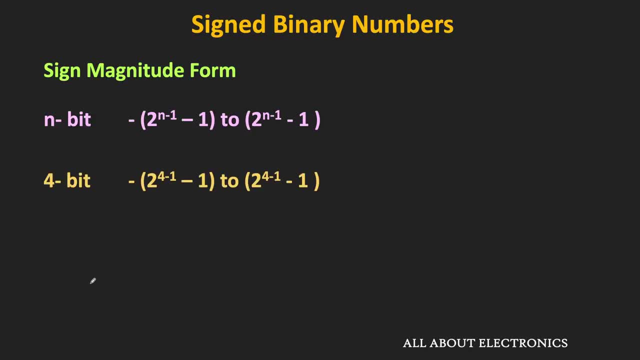 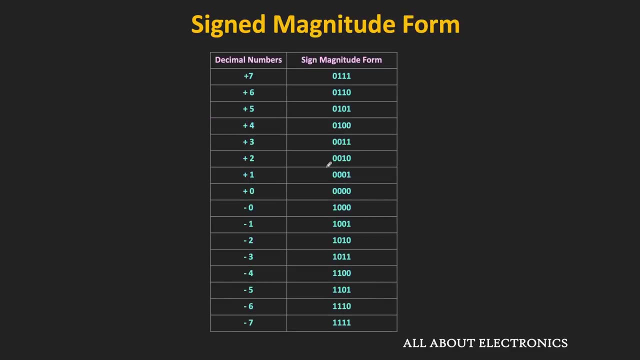 For example, using the 4 bits, the range of number which can be represented are from minus 7 to plus 7.. That means there are 7 negative numbers, 7 positive numbers and 2 different representation of the 0.. Now, although the representation of this sign number is pretty straightforward, in this sign, 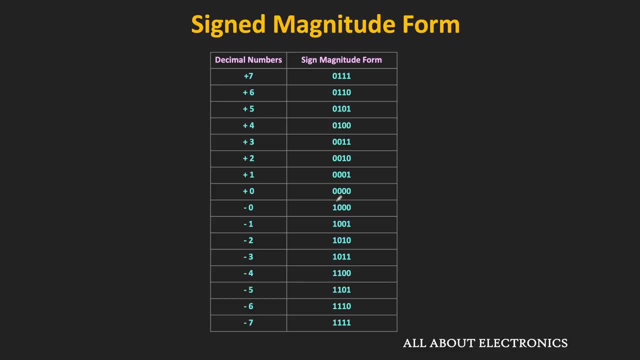 magnitude form, but if we perform the arithmetic operation in this particular form, then it requires a great deal of manipulation. Moreover, there are two different representations of 0. And therefore the use of this sign magnitude form in the digital circuits and the computer. 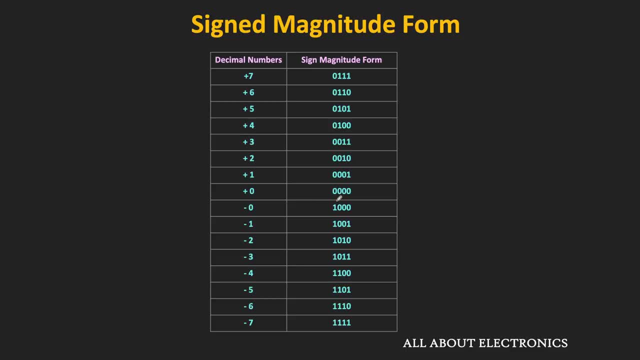 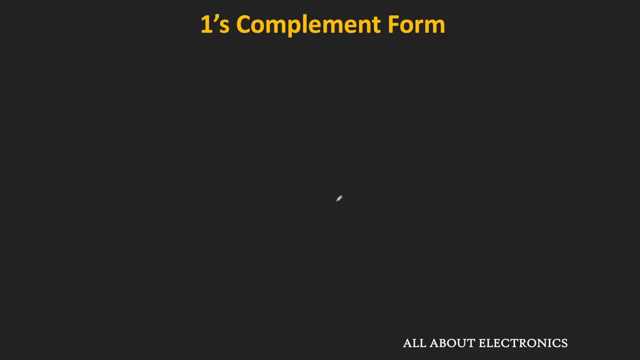 is a bit impractical. Alright, so now let's see the once-complement representation. So, as I said earlier, In this once-complement form the representation of the positive number is same as the sign magnitude form. That means the magnitude of the number is represented in the true binary form. 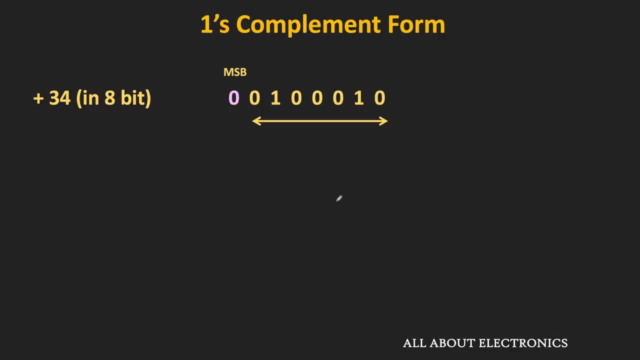 And for the positive number, this msb is equal to 0.. But the representation of the negative number is bit different. So to represent the negative number in a once-complement form, first of all just write the equivalent positive number. So in this case, 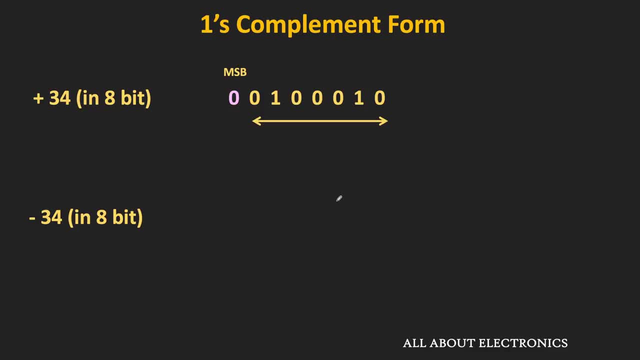 Suppose, if we want to represent the minus 34. Then we have to write the equivalent positive number. If we want to represent the minus 34 in a once-complement form, then first of all let us write the equivalent positive number And now in that number just invert the zeros with the 1 and ones with the 0.. 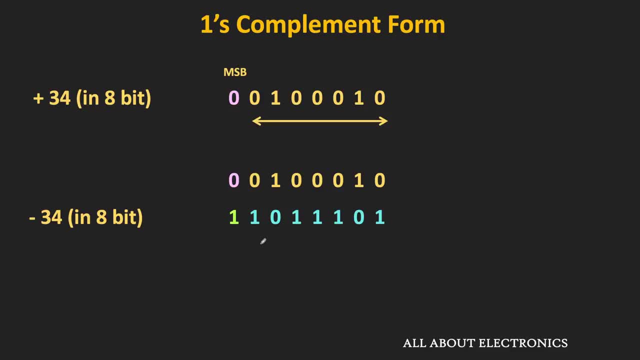 And in this inversion also include the sign bit. So this represents the minus 34 in a once-complement form And in fact it is called the once-complement of the plus 34.. That means just by inverting the ones with the zeros and zeros with the 1 in the positive. 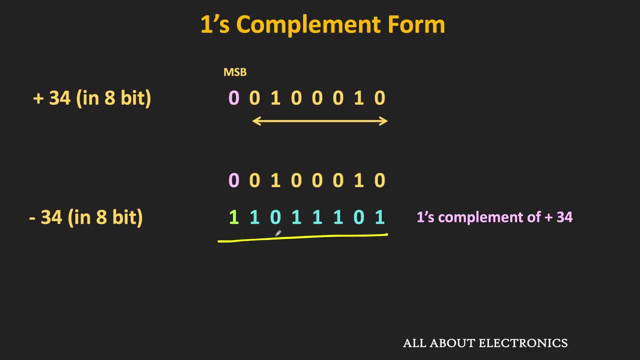 number, The travelling number. at I and N we can find the once-complement of that particular number. So let us understand how it works. So mathematically, for some N bit number N, It's once-complement is equal to 2 to the. 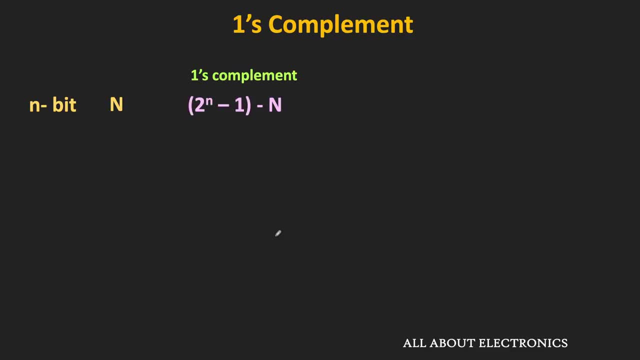 power N-1 minus N. So for example, let us take one number: 12.. So if we represent it in a 5 bit form, then it is equal to 01100, and its once-complement is equal to 2 to the power 5 minus 1 minus N. 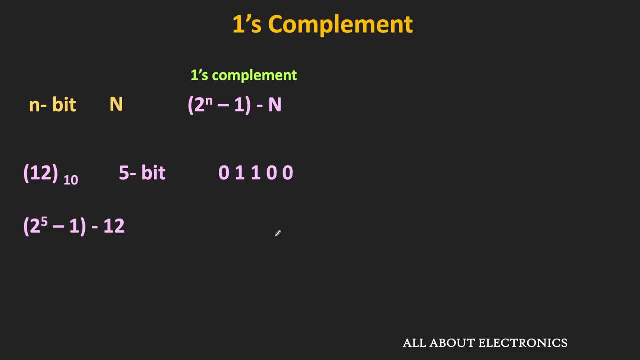 So take a balance. this: Why this is true? Why not? So, in a binary form, this is how it can be represented. So if we subtract this 12 from the 31,, then we will get 10011.. That means the 1's complement of this 12 is equal to 10011. 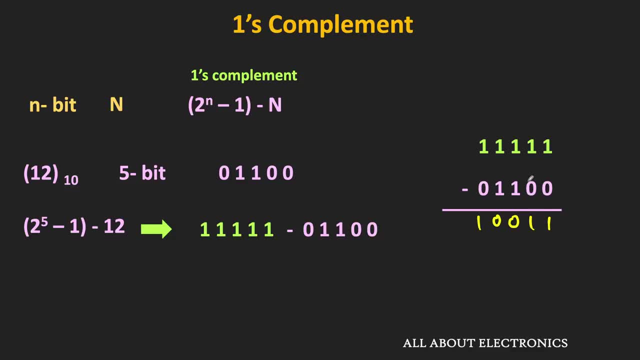 So, as you can see, whenever we subtract a number from all 1's, then 0 in that number will get replaced by the 1, while the 1 in that number gets replaced by the 0. That means, in the given number, if we replace all the 0s by 1 and 1s by 0, then we can directly. 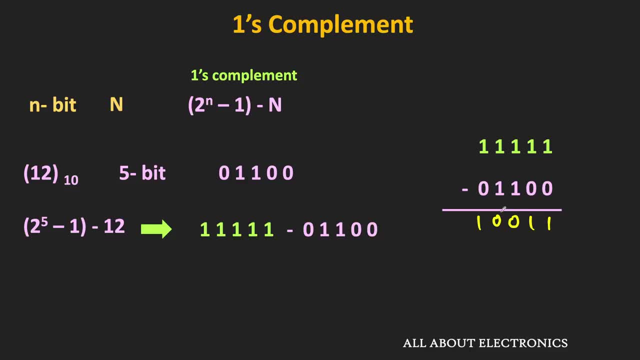 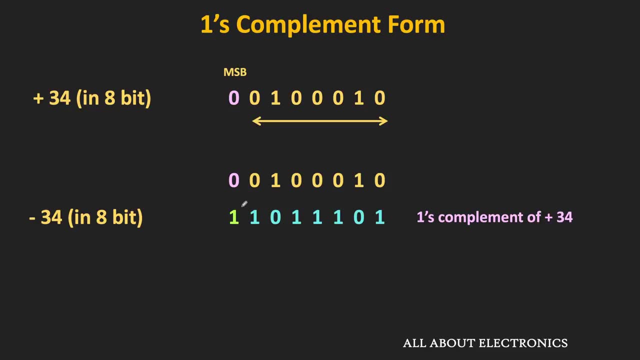 find the 1's complement of that given number. So, as we have seen, the 1's complement of the positive number is equal to negative number. So after the 1's complement, this 0 in the MSB gets replaced by the 1,, which indicates: 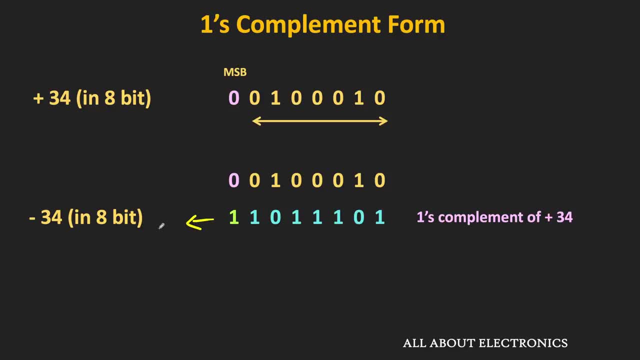 that after the complement the number gets replaced by the 1.. And if we once again take the 1's complement of this number, then once again we will get the original number. That means, in this number if we replace all the 1s by 0 and 0s by 1,, then once again we 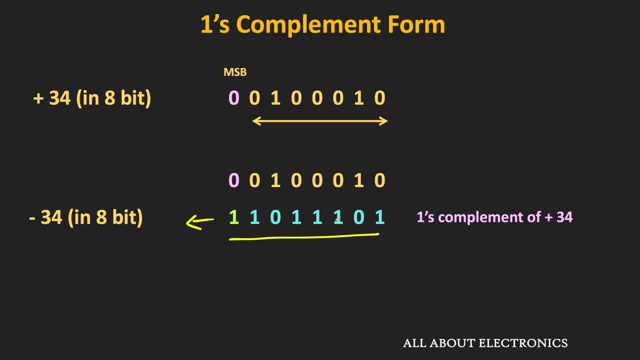 will get our original number. So that is how we can perform the 1's complement of the given number. So, using n bits, the range of number which can be represented in this 1's complement form are from: For example, using 4 bits, we can represent the number starting from: 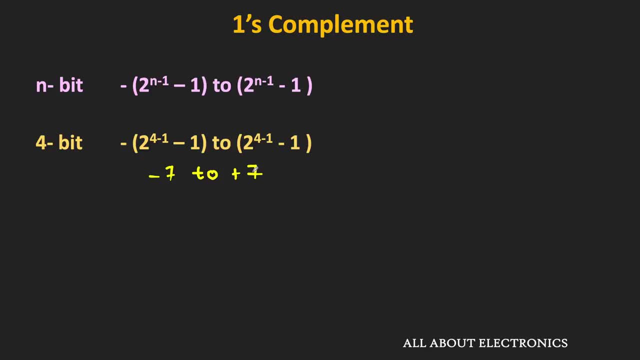 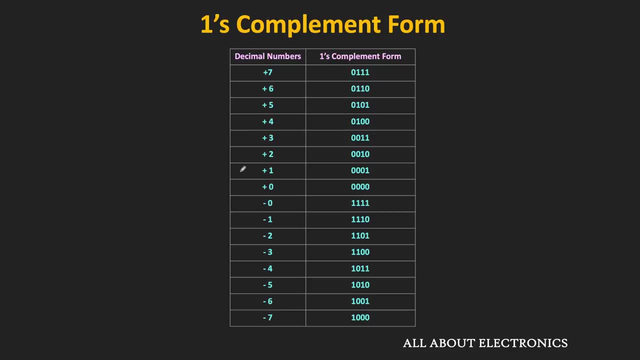 And here is the list of all numbers which can be represented in a 1's complement form using 4 bits. So here, as you can see, similar to the sign magnitude form, there are two different representations for 0.. Now from the digital hardware perspective. 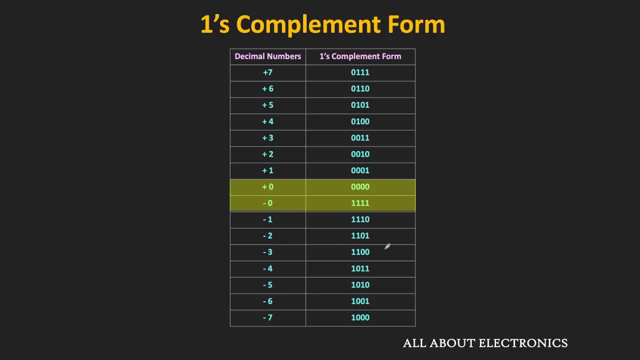 Finding the 1's complement of the number is very easy Because simply, we need to replace all 1s by 0s and 0s by 1 in the particular number right. So even using simple NOT gate, we can find the complement of the given number. 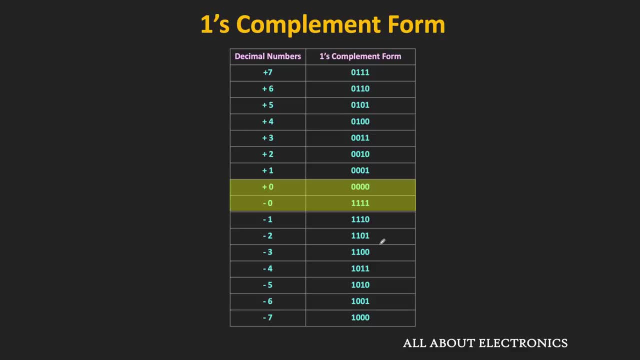 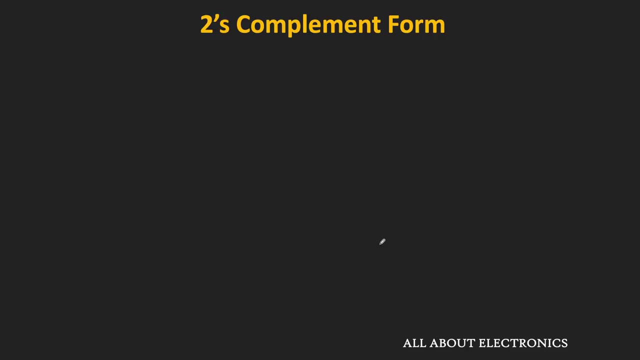 But the only disadvantage of this 1's complement form is that there are two different representations for the 0. So that is all about the 1's complement. Similarly, now let's see the 2's complement representation. So in the 2's complement form the representation of the positive number is same as the 1's. 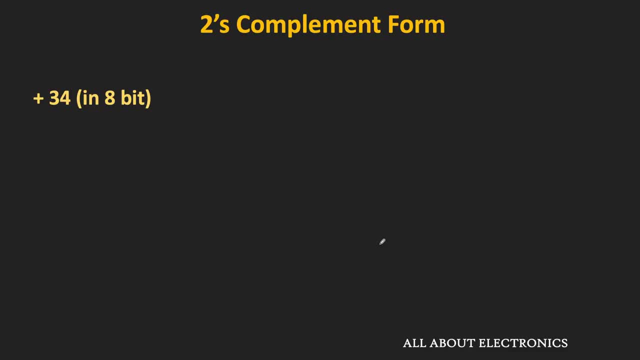 complement and the sign magnitude form. That means for the positive number, the MSB or the sign bit is 0 and the magnitude is represented in a true binary form. And if we find the 2's complement of that positive number then we will get the equivalent. 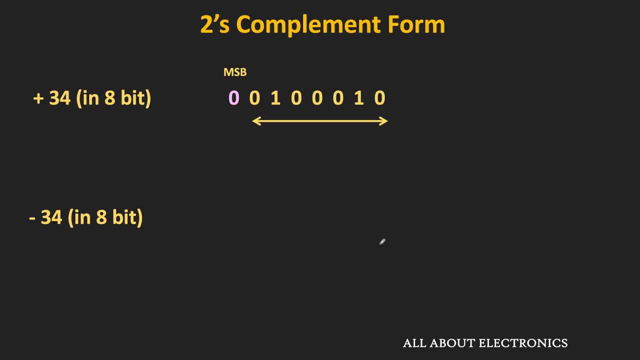 negative number in the 2's complement form. For example, if we find the 2's complement of this plus 34, then we will get the minus 34.. Or, to be precise, we will get the 2's complement representation of this minus 34.. 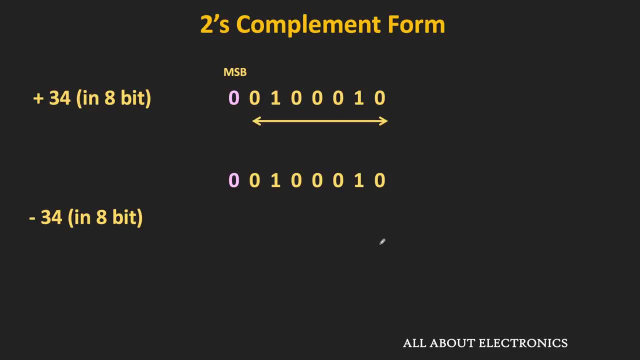 So there are a couple of ways for finding this 2's complement. So if you want to represent the minus 34 in a 2's complement form, then first of all write down the number corresponding to plus 34.. So in the 8-bit form it is equal to 0010010.. 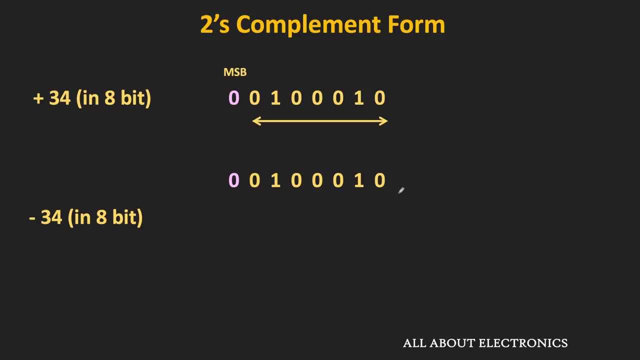 Now, starting from the least significant bit, or the LSB, Copy all the bits Until you encounter the first one. That means copy all the bits up to first one And then, after, replace all 0's by 1 and 1's by 0, including the sign bit. 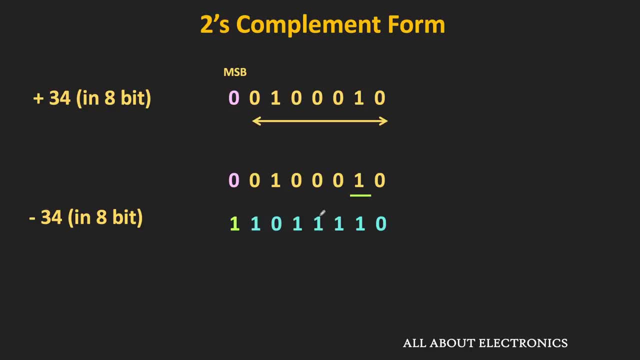 So, after the first one, all the 0's have been replaced by the 1 and 1's have been replaced by the 0. So this representation is a minus 34 in the 2's complement form, Or in other words, it represents the 2's complement of the number plus 34.. 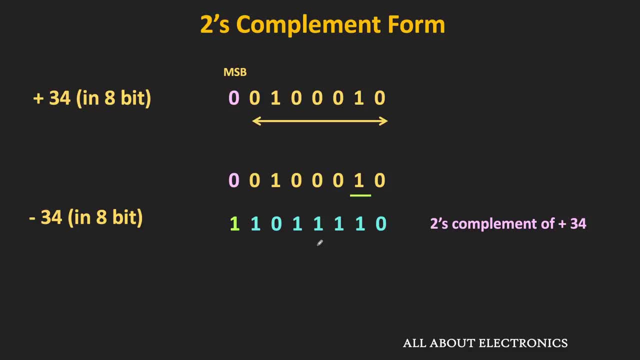 So this is one way of finding the 2's complement of that number. The second way is First take the 1's complement of that number And then add 1 to the 1's complement, So the resultant is the 2's complement of that particular number. 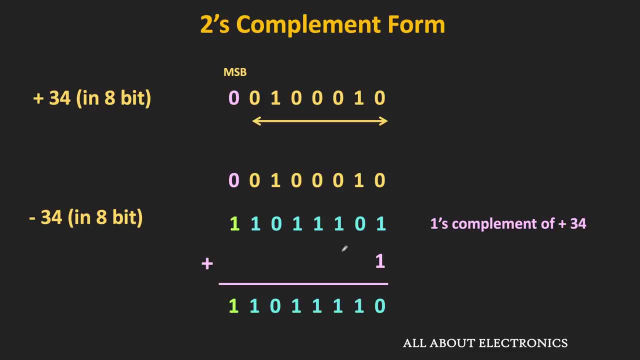 So, as you have seen earlier, For finding the 1's complement We need to replace all the 0's by 1. And 1's by 0 in that particular number, And then after, if we just add one to the 1's complement, 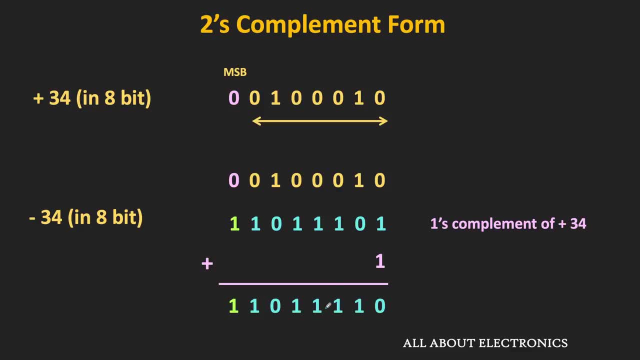 we will get the 2's complement of that particular number. So in this case, by this method, we will find the 2's complement of the number plus 34.. So this is the second way of finding the 2's complement of that particular number, And the third one is the traditional way. So, mathematically, 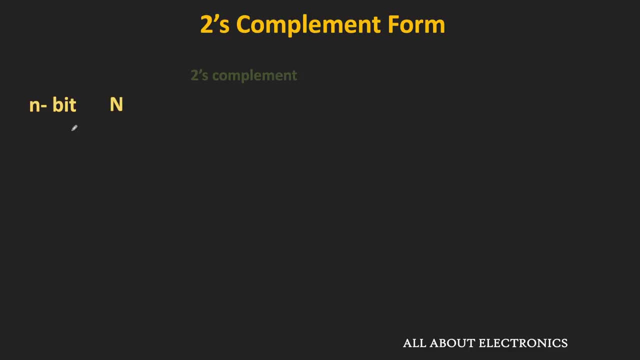 if we have some n bit number n, then its 2's complement is equal to 2 to the power n minus n. So once again, let us take the number 34.. And this is how it can be represented in a 8-bit form. 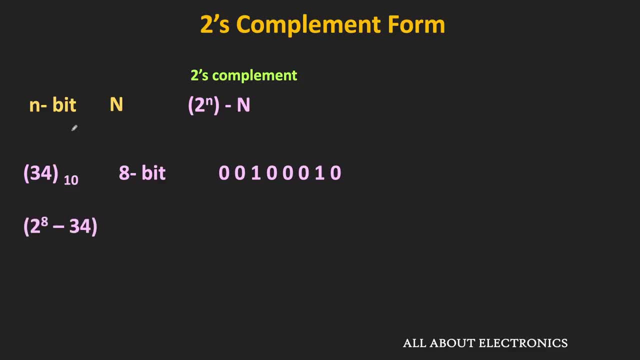 So its 2's complement is equal to 2 to the power 8 minus 34.. Or in a binary form, it is the subtraction of the number 256 and 34.. So if we do the subtraction, then we will get a number that is 110 00, 100,, which is the 2's complement of the number plus 34.. 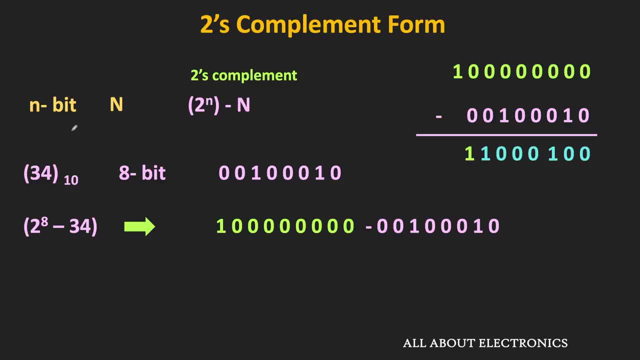 So this is the another way of finding the 2's complement. Now here, this 2 to the power n minus n can also be written as 2 to the power n minus 1 minus n plus 1.. So here, if you observe, then this: 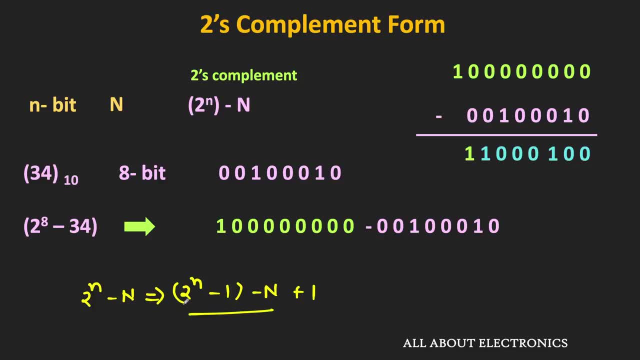 2 to the power. n minus 1 minus n is actually a 1's complement of the number n. Therefore, if we just take the 1's complement of the number n and if we just add 1 to it, then we will get. 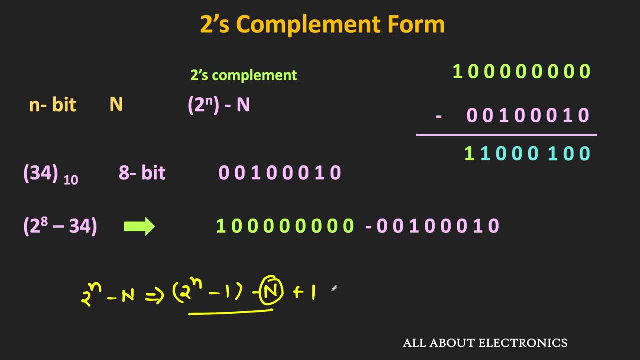 the two's complement of the number n. So to find the two's complement of the number, you can follow any of the three methods, But the first one, which I have discussed earlier, is more convenient for the hand calculations. Alright, so now let's take one more example. 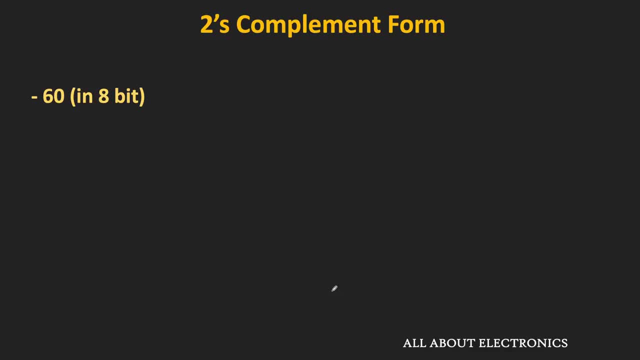 So let's say we want to represent this minus 60 in the two's complement form. So first let us write down the number corresponding to plus 60.. That is equal to 0, 0, 1, triple 1, double 0.. 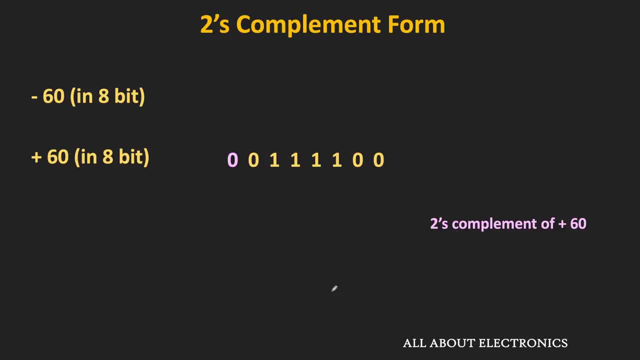 Now to find the two's complement of that number, starting from the LSB, just copy all the bits until you encounter the first one, And once you encounter the one, then after that replace all the zeros by the one and ones by the zero in that particular number. 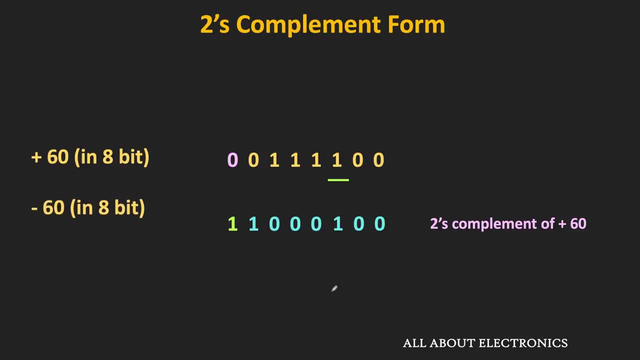 So this is the representation of the minus 60 in the two's complement form. So in this way we can find the two's complement of the given number. Now using the n bits, the range of the number which can be represented in this two's complement form. 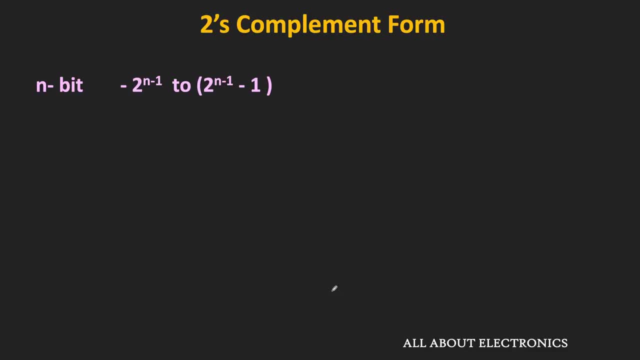 are from minus 2 to the power n minus 1 to 2 to the power n minus 1 minus 1.. For example, using the 4 bits, we can represent the numbers starting from minus 8 to plus 7.. So here is the. 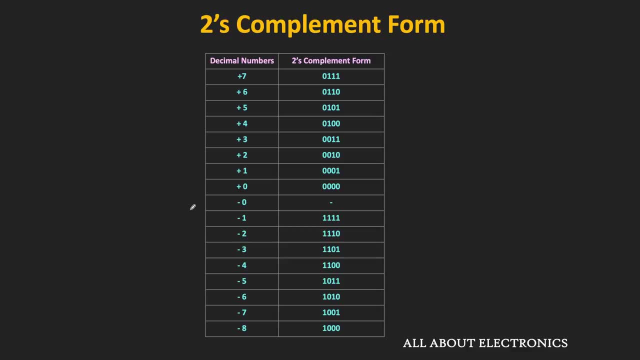 list of all the numbers which can be represented using the 4 bits in the two's complement form. So using the 4 bits we can represent 7 positive numbers and 8 negative numbers, And in this two's complement form there is only a unique way of representing this zero. So if we take the two's 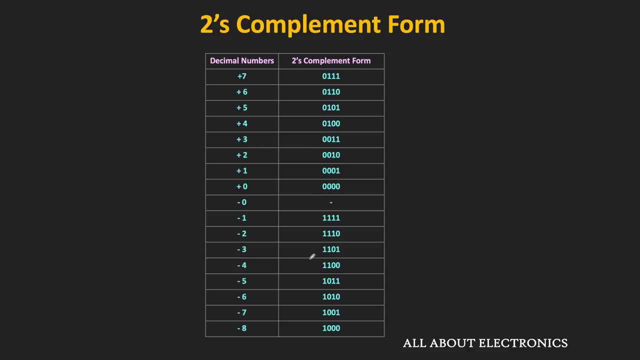 complement of this number plus 3,, then we will get the minus 3.. Likewise, if we take the two's complement of the negative number, for example a minus 5,, then we will get the positive number. But if we try to find the 2's complement of the most negative number, then we will 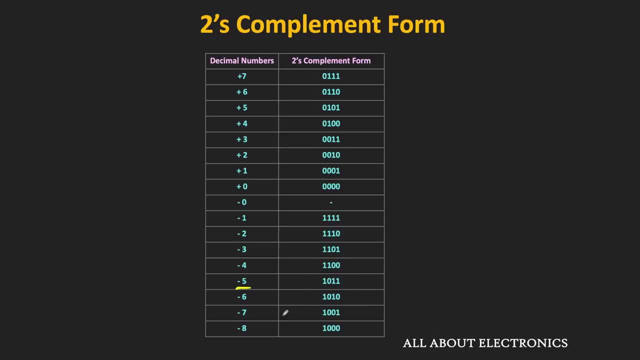 get the same number. For example here: if we try to find the 2's complement of the number minus 8, then we will get the same number. The reason is that in this 2's complement form we can represent one more negative number. 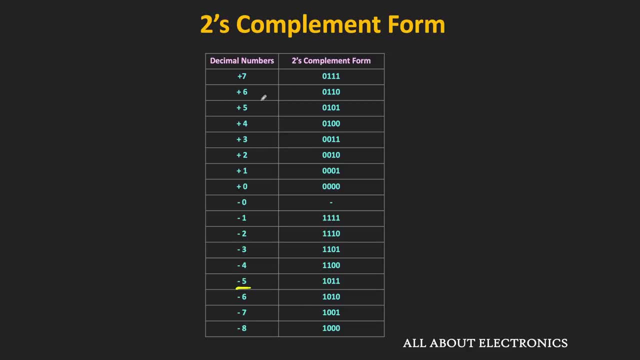 than the positive number. So if we try to find the 2's complement of this most negative number, then there is no corresponding positive number in this representation. That means if we try to find the 2's complement of this most negative number, then we will. 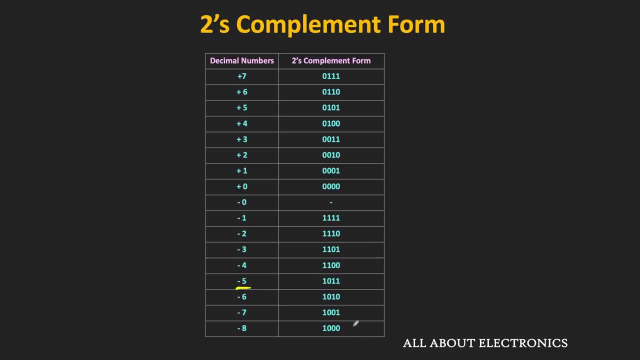 get the same number. So that is one more thing which we need to keep in mind while performing the 2's complement. So, as I said, this 1's and the 2's complement, and specifically this 2's complement, is very 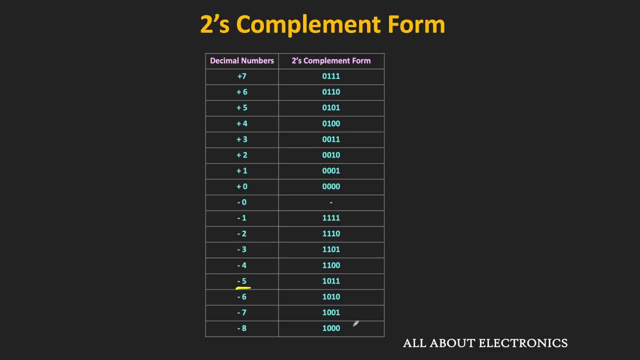 useful in performing the arithmetic operations Because with the 2's complement representation without using the subtraction circuit, it is possible to perform the subtraction only using the header circuit. So in the next video we will see that how to perform the binary addition and the subtraction.